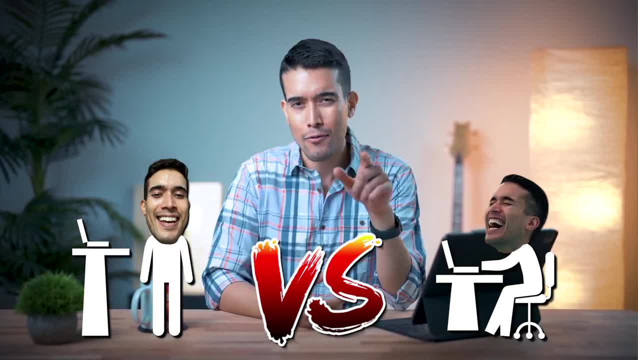 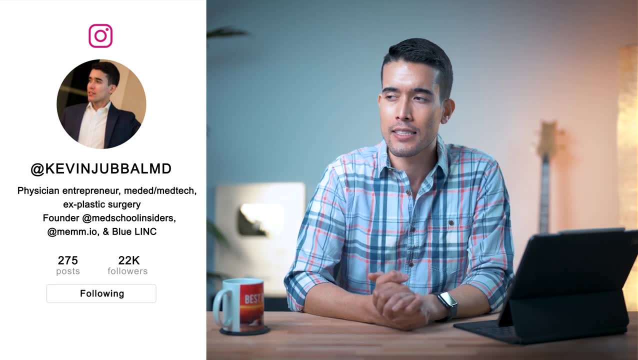 You've heard, standing desks are all the rage, but are they actually better than regular sitting desks? Let's find out What's going on, guys. For those of you who are new here, my name is Kevin Jubbal, physician entrepreneur based in Las Vegas. Now, I made a previous video called 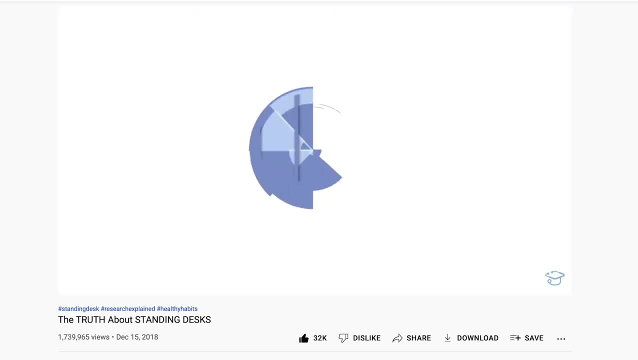 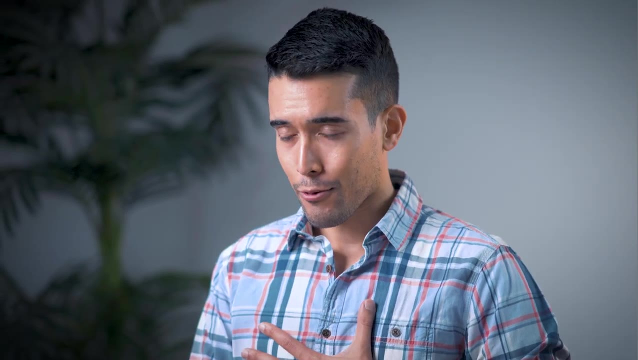 The Truth About Standing Desks on the Med School Insiders YouTube channel. In this video, we're going to dive into some of the aspects I did not cover in that video, including treadmill and bicycle desks, as well as a few other factors. So as for my background with standing desks, 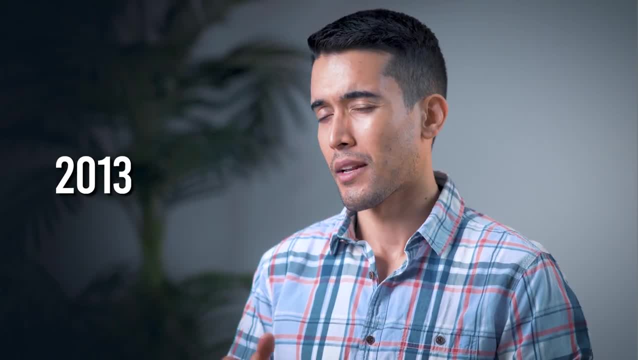 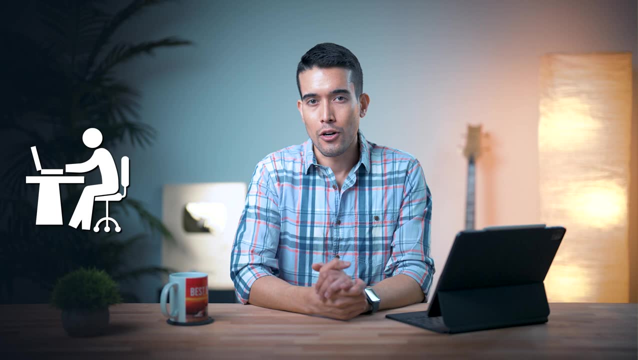 I started using a standing desk back in 2013,- so it's been about nine years, And that was a fake standing desk. I purposely did not even have a stool nearby. However, a few months ago I changed to a motorized sit-stand desk and I actually have a whole office tour that you can. 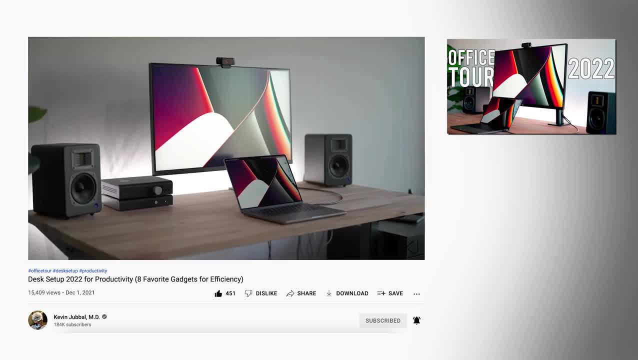 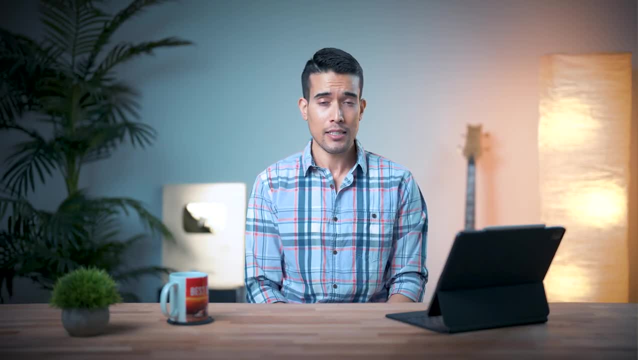 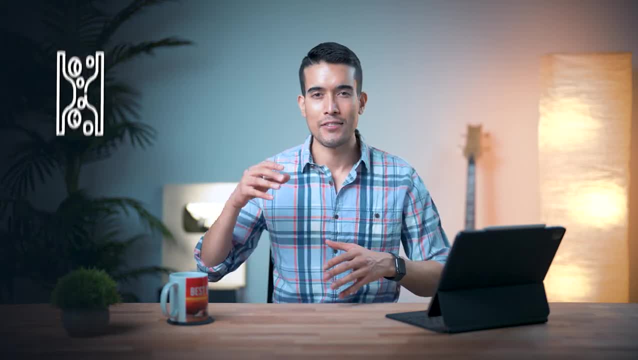 It essentially boils down to being sedentary. It essentially boils down to being sedentary is bad, And I'm not going to bore you with all the details about the rate of DVTs versus stroke, versus diabetes, yada, yada, yada. Well, for two reasons: Number one, I'm going to bore you, And number two: 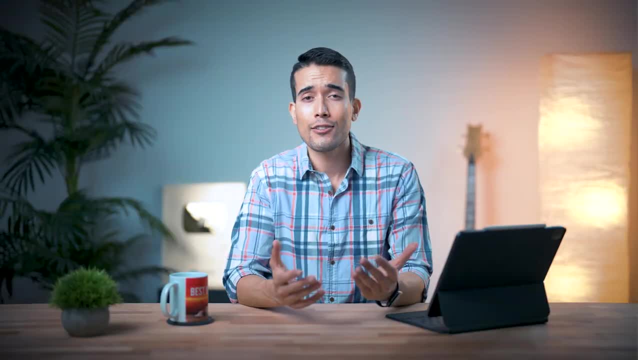 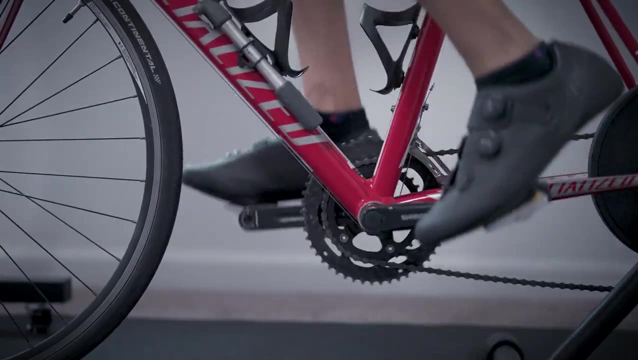 a lot of it is very weak correlational research And you may say, hey, I exercise one hour per day, five days a week. I'm good, I don't need to worry about the negative effects. Not quite. Exercise, even if you are very regular with your exercise, is not going to completely reverse all. 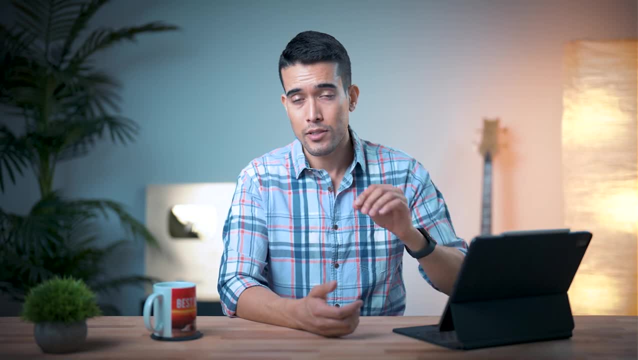 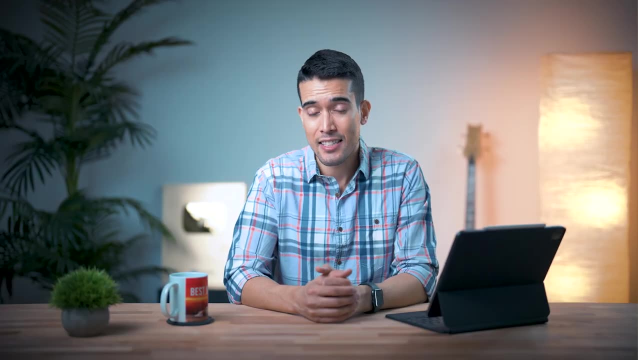 those negative effects of sitting for eight plus hours a day And also sitting for prolonged periods really increases the pressure on your lower back and you tend to have more back issue issues when you're sitting a lot. It's actually one of the main reasons that I hate sitting too. 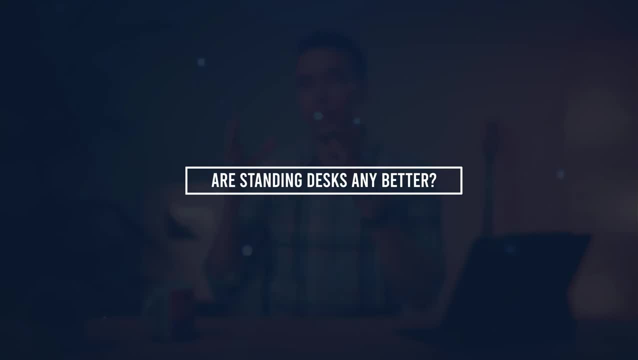 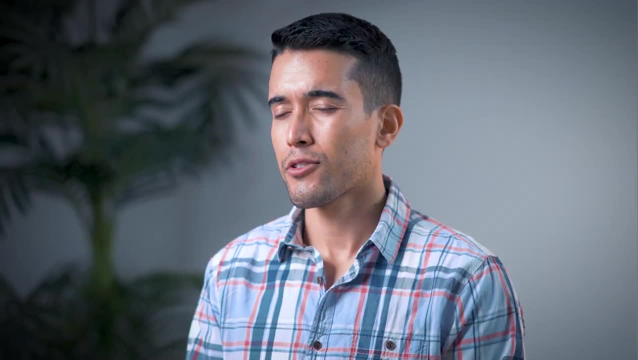 long, But are standing desks any better. So the logic being that, hey, if we're sitting for too long, then maybe we should be standing at our desks. That's going to force us to move, maybe a little bit, and that's going to be better. At least that's the logical reasoning. But there's 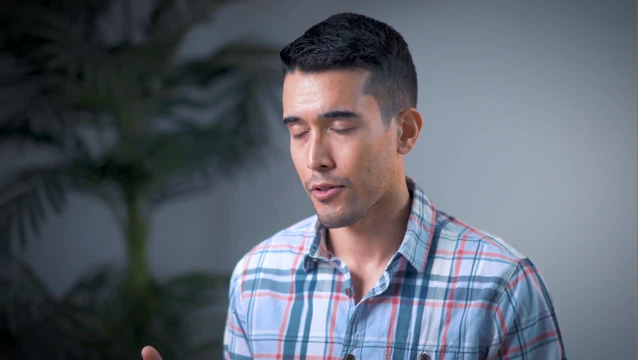 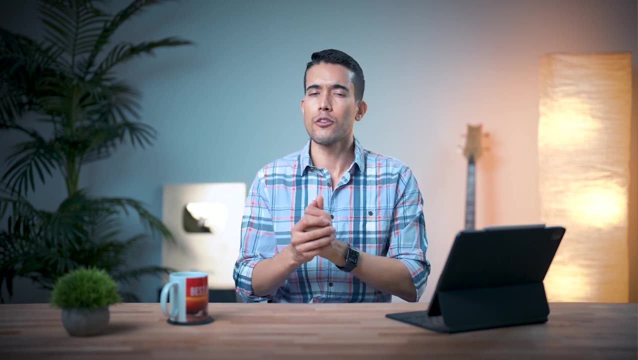 some conflicting evidence as to whether standing is actually any better. For example, people talk about glucose variability And some studies will say that reduced glucose variability results from standing, which is a good thing, And others will say, nah, no difference. Another example is some 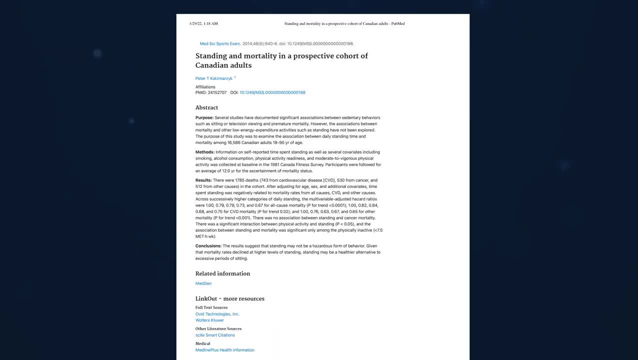 studies will report an increased association with morbidity And some studies will say that if you reduce morbidity and mortality from standing, others will have a reduced rate And I know as a viewer this will just frustrate you like. come on, just give me the answer. 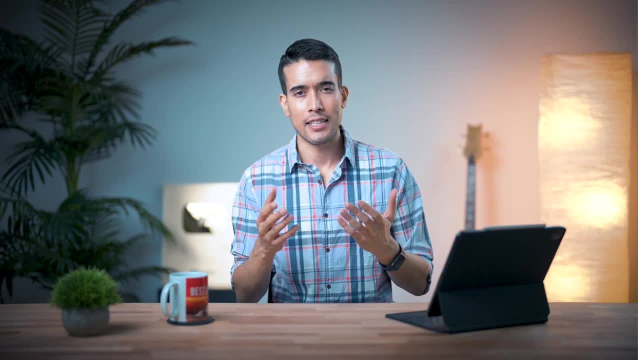 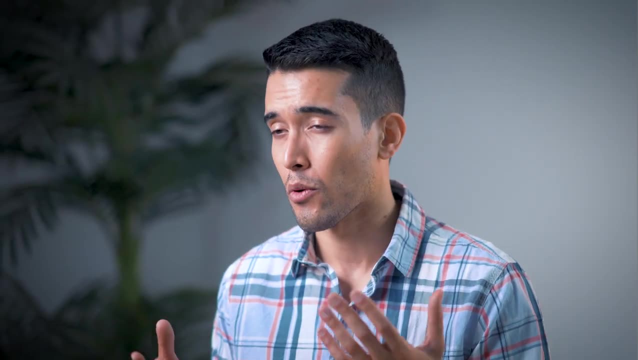 The issue with the research in this area is it tends to be more epidemiologic in nature. It tends to rarely be randomized, controlled trial, blinded, those kinds of things. So you tend to have pretty weak evidence one way or the other And you need to use more clinical judgment. So 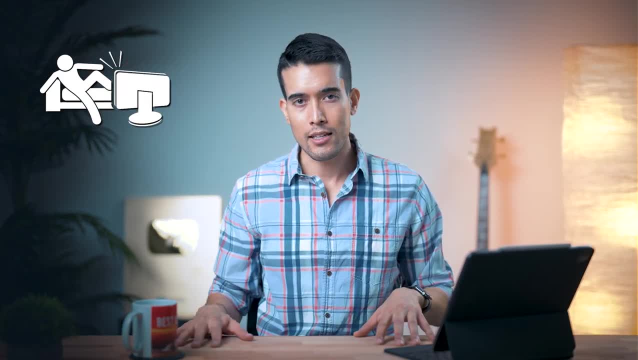 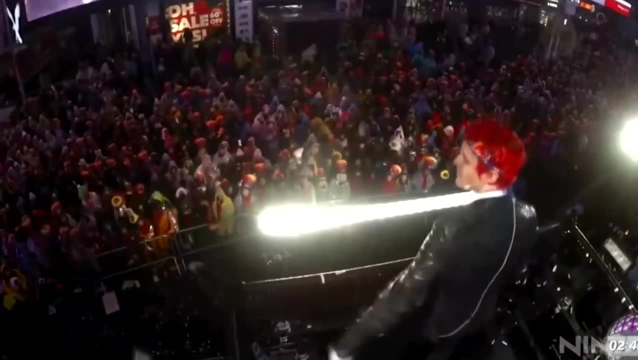 to summarize the research, what we do actually know is being sedentary for too long is bad, Sitting for too long, standing too long- they're both bad. Movement is good. I'm not seeing enough movement, And this is why I believe that a sit-stand motorized desk is actually the best of both. 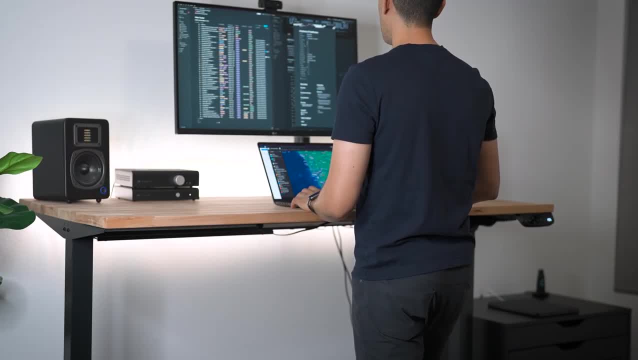 worlds Because you can stand, and when you're standing you tend to move around a little bit more. you're shifting your weight, maybe you're rolling on a lacrosse ball, like I normally do, And then, when you get tired, when your posture starts deteriorating, you start having 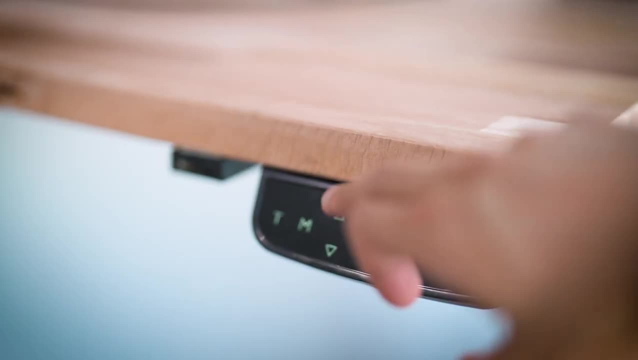 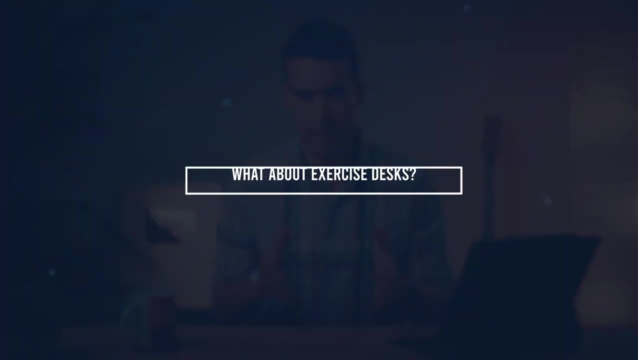 foot pain or whatever. then you can press a button, go back to sitting and then vice versa, Once you are tired of sitting, you start having some lower back pain. you press the button, you go back up to standing. All right, so what about exercise desks? I'm 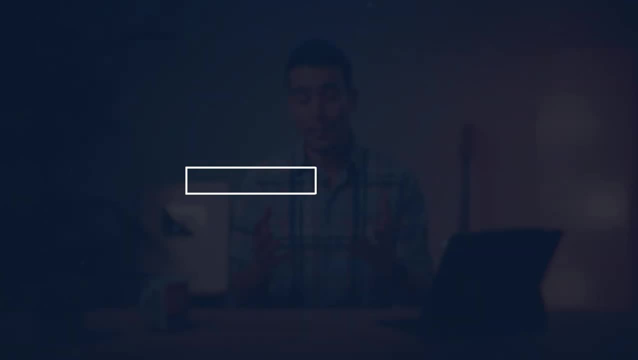 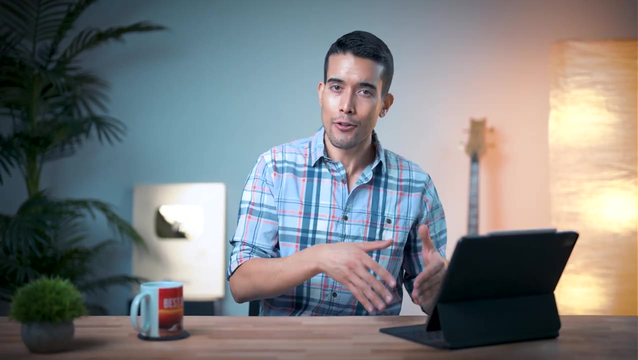 talking about treadmill desks, bicycle desks, things of that sort. Again, research here is conflicting. I found a handful of studies that reported no negative effects on things like typing speed at low intensity cycling, and then other studies that said, yes, there is definitely a negative effect even with low intensity cycling. 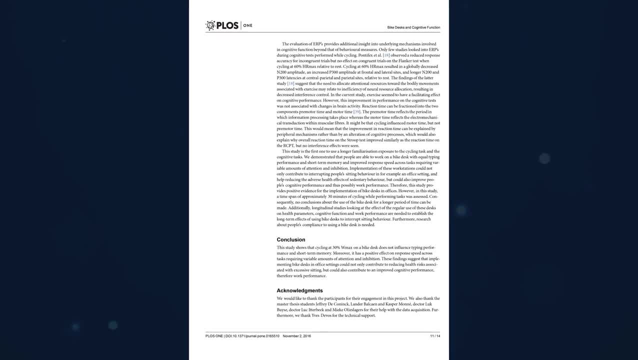 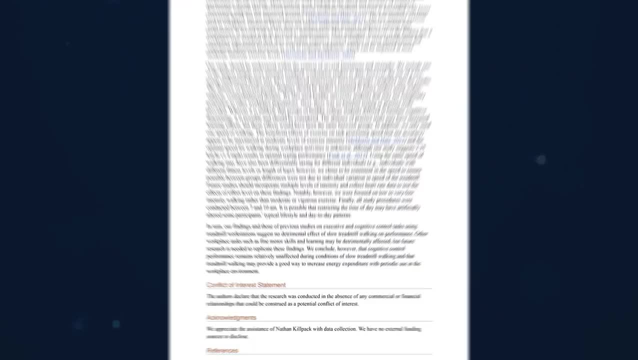 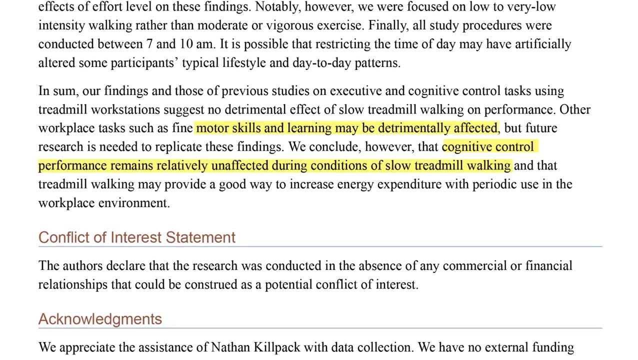 So Torbanes and colleagues in 2016 found a positive effect on speed across tasks requiring variable amounts of attention and inhibition. On the other hand, Larson and colleagues in 2015 found no negative effect of treadmill desks on executive and cognitive control tasks using treadmill workstations, but reduced performance on fine motor skills. 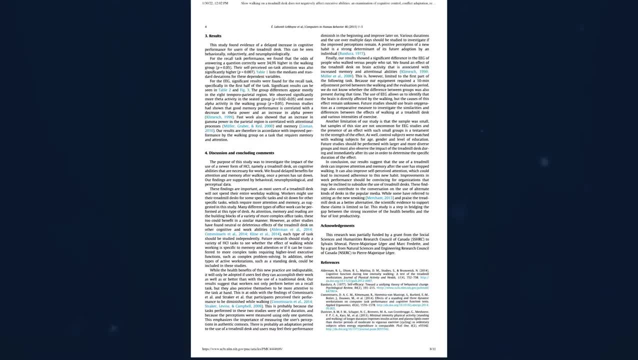 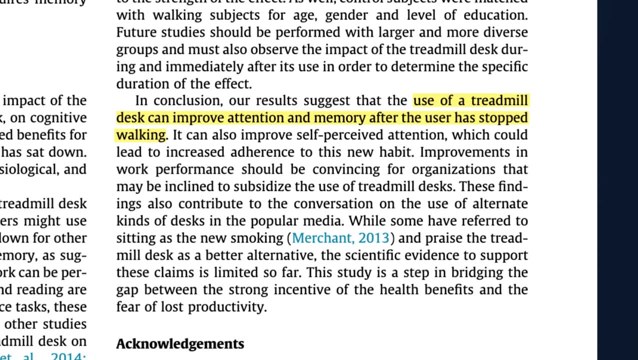 and learning, La Bonte Le Moyne in 2015 demonstrated that you benefit cognitively after using a treadmill desk, not during, And they demonstrated this with cognitive tasks, EEG and participants also perceived themselves to be more attentive. self-reported. 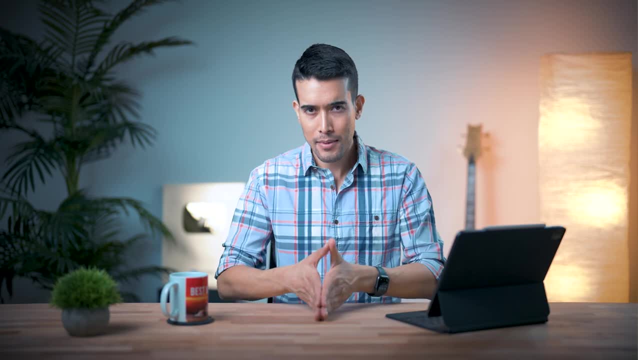 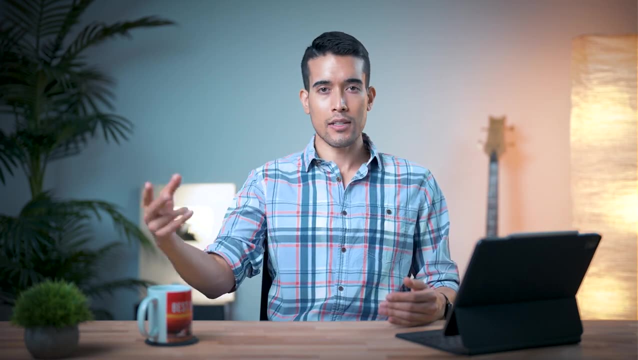 Now the question arises with this finding Okay, was it using the treadmill desk and working on some tasks that then boosted performance after getting off the treadmill desk? or would any physical activity walking outside at a relaxed pace also have the same positive effect? And if? 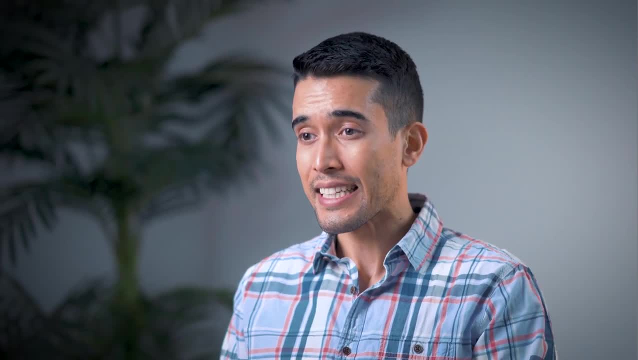 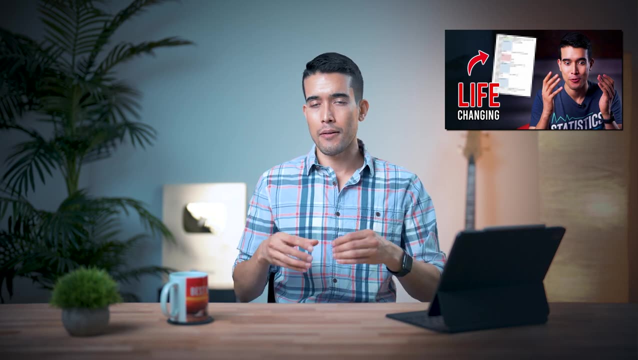 so, then, should we consider using treadmill desks to improve the performance of our work? Should we prioritize people working on more cognitively demanding tasks immediately after walking or getting some light level of exercise? Now? I've actually talked in a previous video about how our brains are wired and better performing at various types of tasks, or 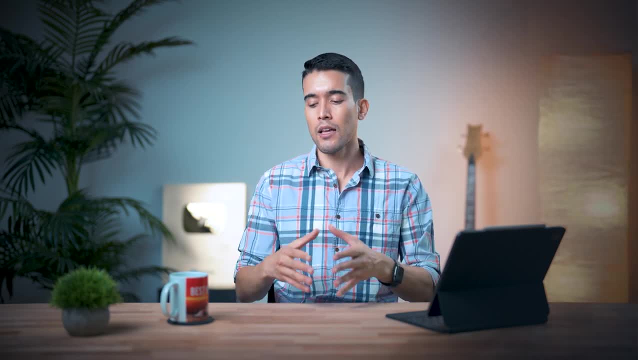 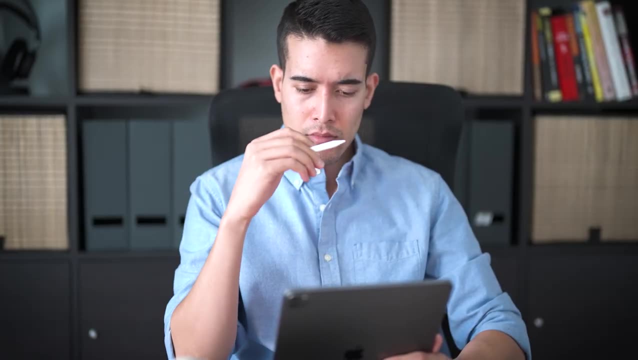 types of mental performance at different times of the day. So for me, for example, the most focused and intense stuff is best in the morning. the more lull in productivity kind of mindless work is best in the afternoon, and then a creative burst occurs in the evenings. 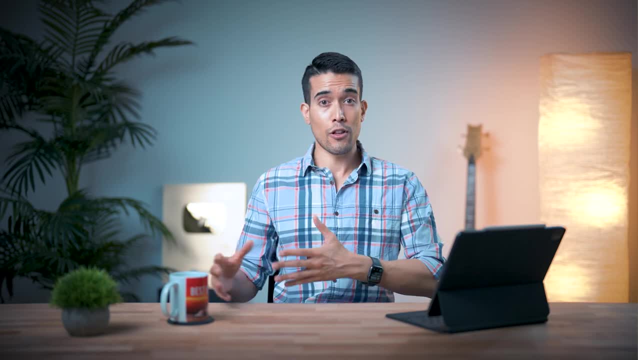 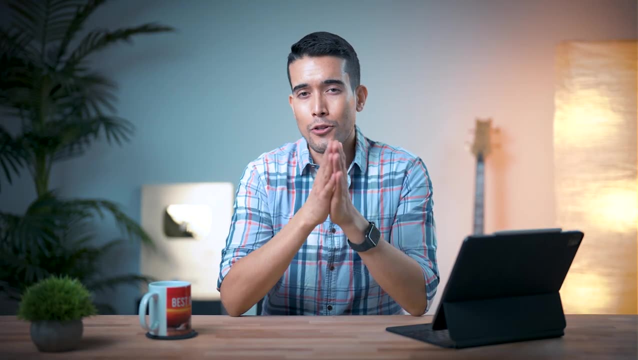 So, knowing this, how can we schedule our exercise, whether a full-on workout or even a brisk walk, at various times of the day to optimize our performance for those cognitive tasks? Now, in summary, when you look at the literature on these exercise desks- and I'm talking treadmill- 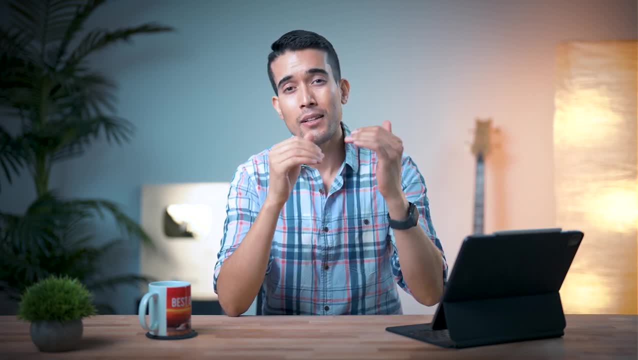 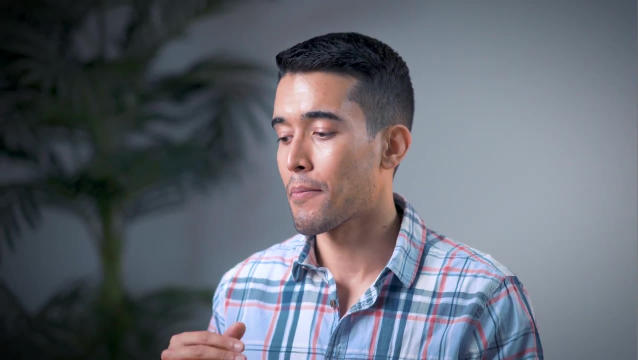 and bicycle desk. they tend to report a zero or minimal detrimental effect on cognitive performance. Very few of them actually report improved performance, And not surprisingly. if you work out at moderate or high intensity, you're going to have more of a cognitive hit. 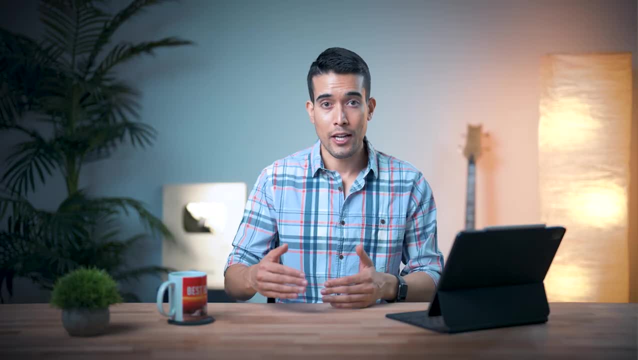 versus working out at a lower intensity. After all, when you are working out at moderate to high intensity, your body needs to allocate more energy to the work that you're doing. Your body needs to allocate more of those resources and energy towards the exercise. 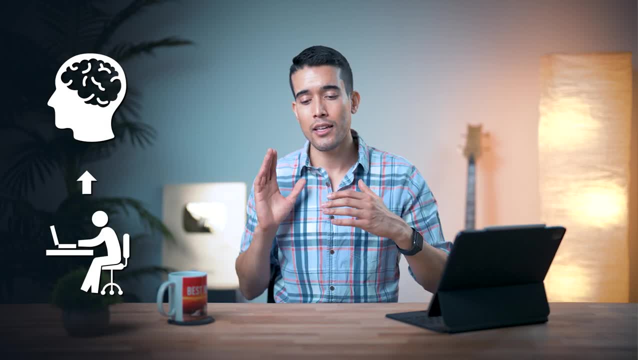 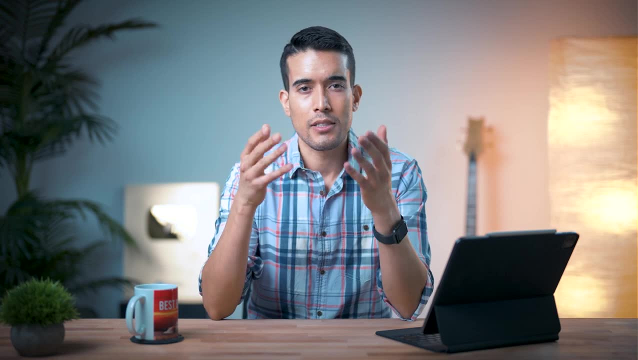 towards your muscles, Whereas when you're at a lower intensity you can then reallocate those resources more for your brain, for neuronal activity. Most studies also suggested using these exercise desks intermittently. right, It's going to help you with increased energy expenditure. 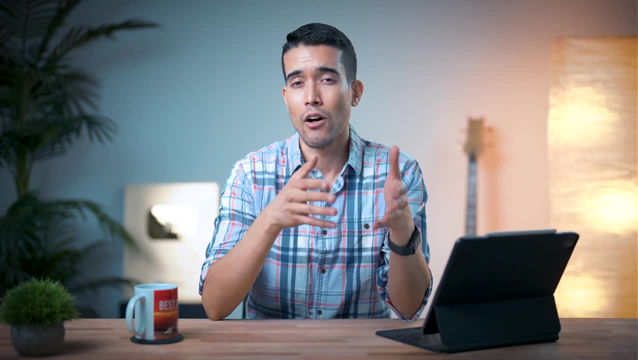 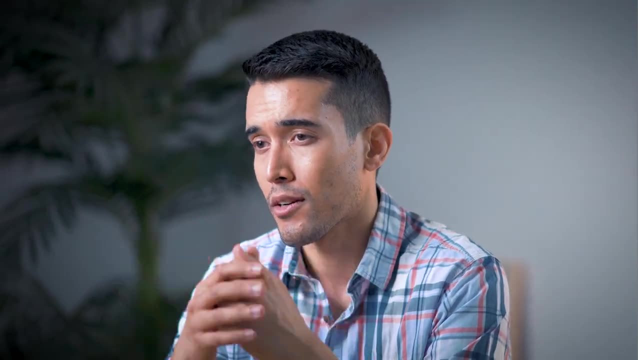 keep you healthier, but they don't actually recommend them as the default, the desk that you want to use day in and day out. My take is, if someone wants to use a bicycle or treadmill desk, then they're probably going to be healthier for it, at least from a cardiovascular and metabolic. 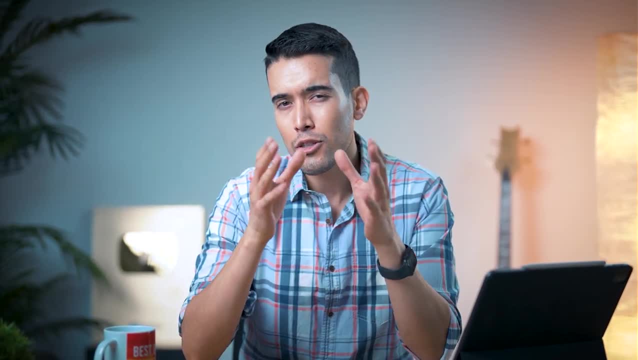 health perspective. So if you're going to be working out at a low intensity, you're going to want to use a bicycle or treadmill desk, which is really important, but you probably shouldn't use it that much during the cognitively demanding tasks- I often talk about batching tasks- to 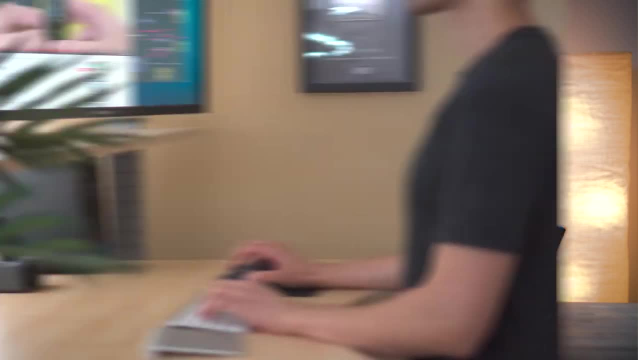 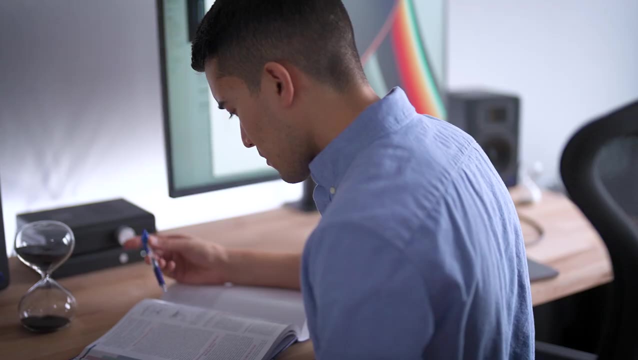 improve your productivity and performance. So if I'm going to spend an hour doing email, that's a great time to use one of these bicycle desks. But if I'm doing something more cognitively demanding- let's say I'm studying for a med school test, or I'm working on a new video script, or 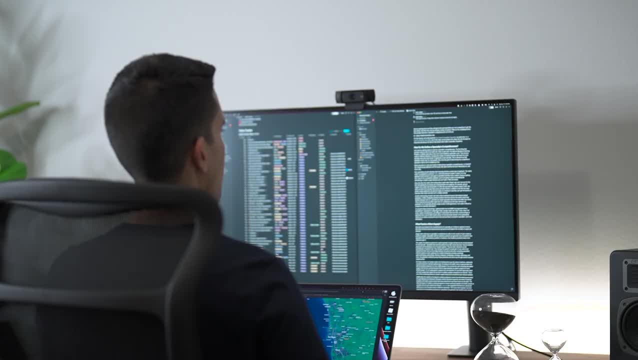 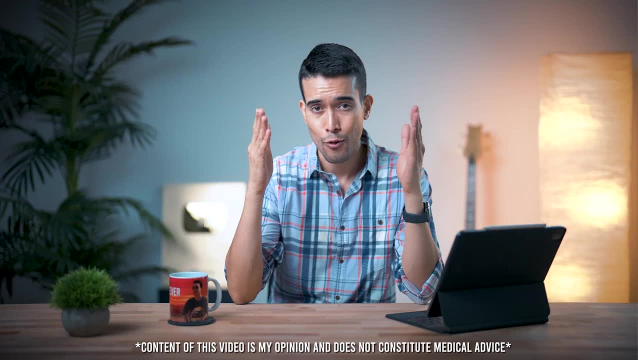 anything else that is more intense, I'll go to my standing or sitting desk. So what should you do? First of all, that decision is up to you and your physician. This video does not constitute medical advice. This is for informational purposes only and no patient. 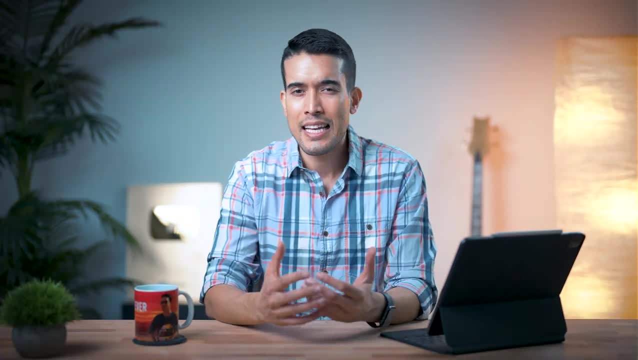 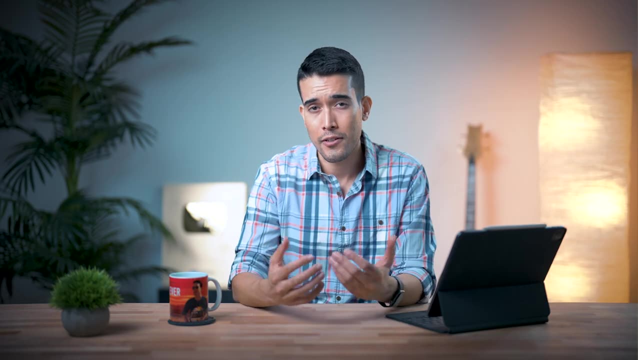 physician relationship is formed. So first of all, research. in this space it kind of sucks. The overwhelming majority of the studies were retrospective in nature and they didn't really do a good job of randomizing or controlling for confounding variables. For example, there's a study from Smith and colleagues and they demonstrated 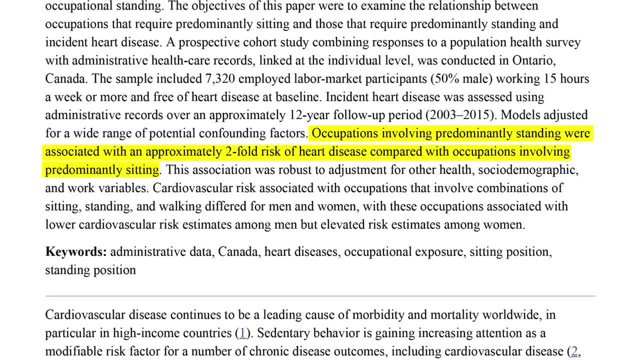 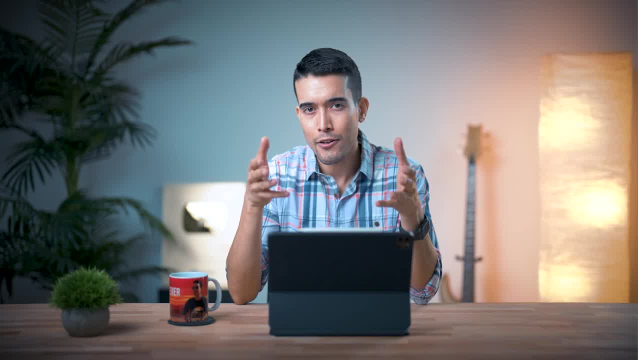 that people with working occupations involving primarily standing were associated with a twofold increase in heart disease. But without for controlling the types of occupations, the various socioeconomic factors and other variables, this isn't really meaningful. The data are quite strong that being sedentary definitely not good for you, But I'm not fully. 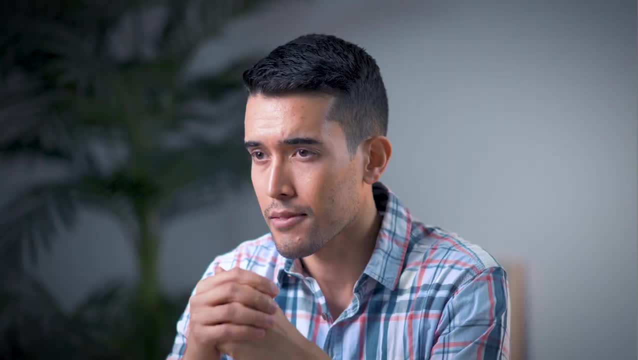 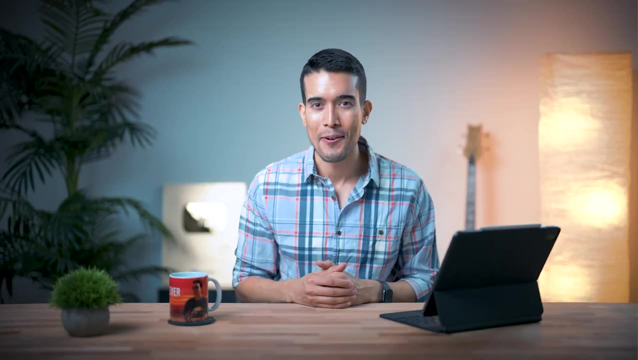 convinced that something as simple as just using a standing desk is the solution. This is a complex problem. People aren't getting that much exercise anymore in their lives And we're hoping for this quick, easy fix, the classic American way right, But unfortunately even with the scientific method. 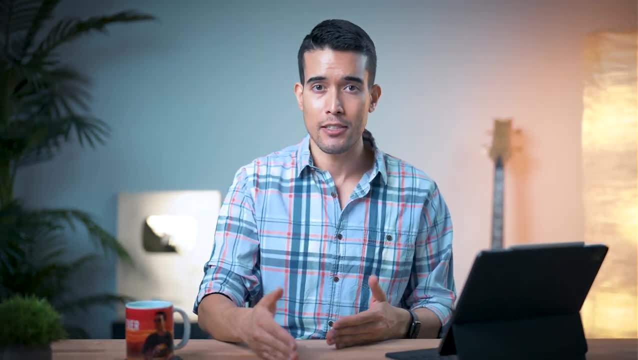 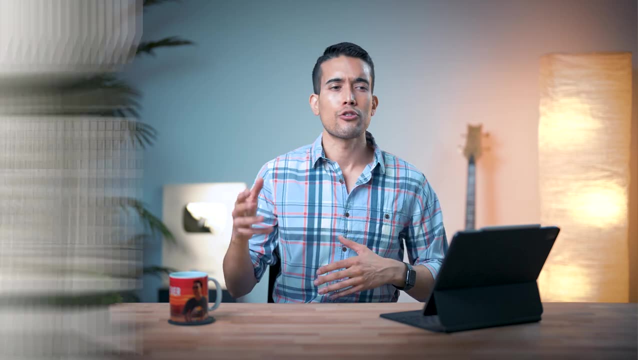 we don't get clear cut answers, We need to make decisions with imperfect information. That's just life. What the literature does say is that standing or sitting for too long they're both problematic. So what you want to be doing is stretching, shifting, moving, walking. 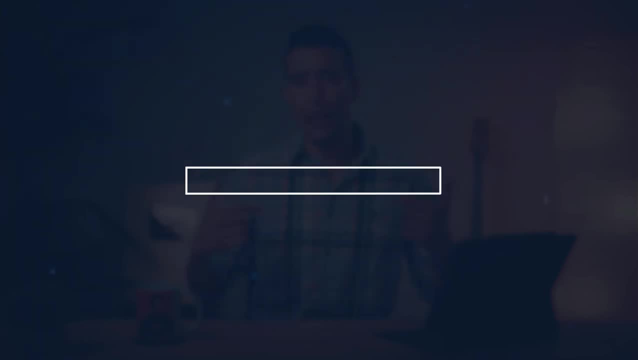 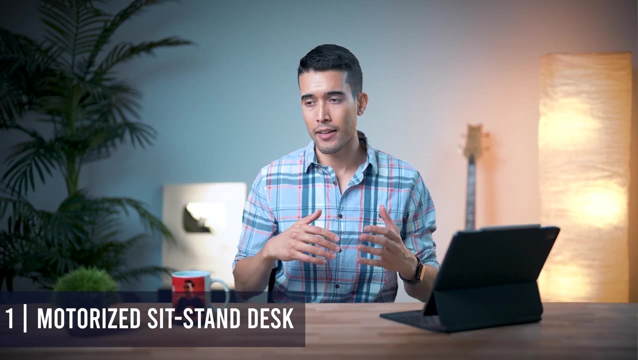 yoga poses, whatever throughout the day. Now, finally, here is what I do, And it comes down to three actionable steps. Now, first up is that a motorized sit stand desk has made an immediate improvement in my physical discomfort, aches and pains throughout the day. And if you're 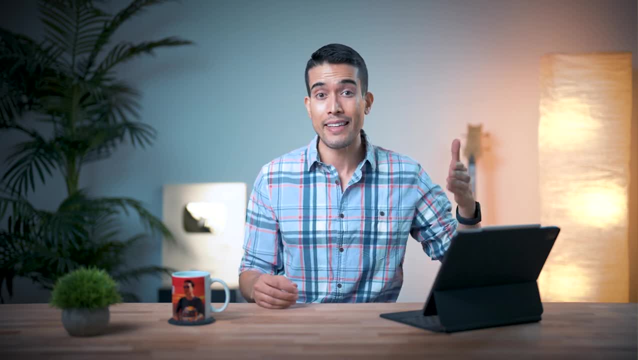 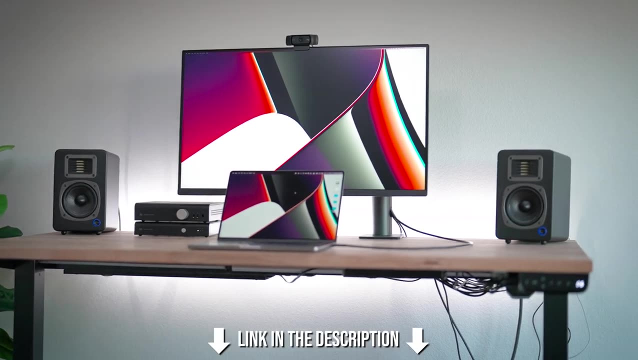 eliminating pain and discomfort. you are immediately becoming more productive. You're becoming less distracted. I actually really like the motorized base that I use. It was like 250 on Amazon. You can attach it to any desk, even something like this, And you can find a link. 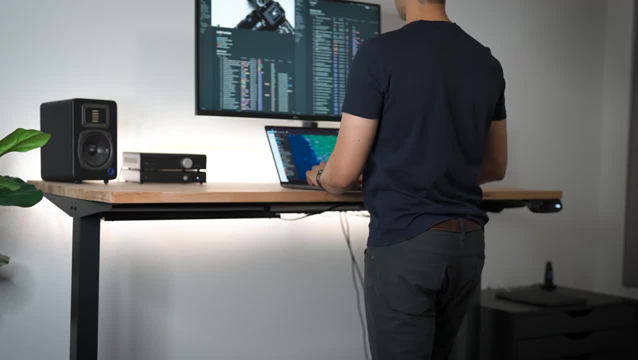 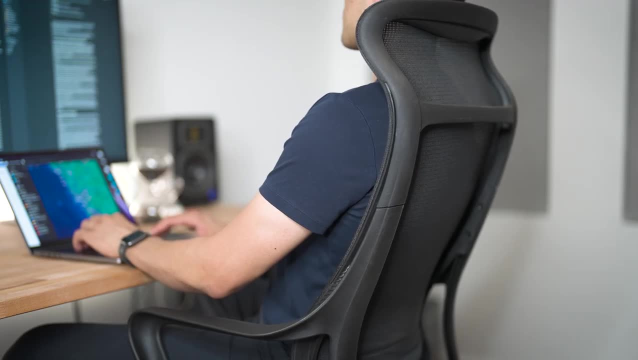 to it down in the description. I start the workday off at a standing position because later in the day I'm going to be too tired. I won't want to do that, And once I get tired, after an hour or two, then I'll press a button, go back down to sitting and rinse and repeat Once I get tired of sitting. 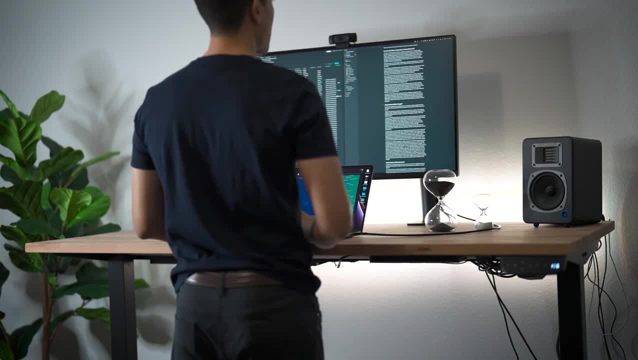 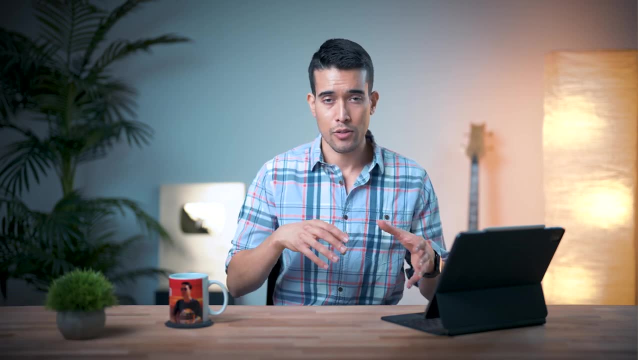 I start noticing some aches and pains or just discomfort anywhere, then press a button and go back up to standing. Number two is I stay hydrated. If movement is the key and not staying at your desk in either a sitting or standing position too long, then simple solution. 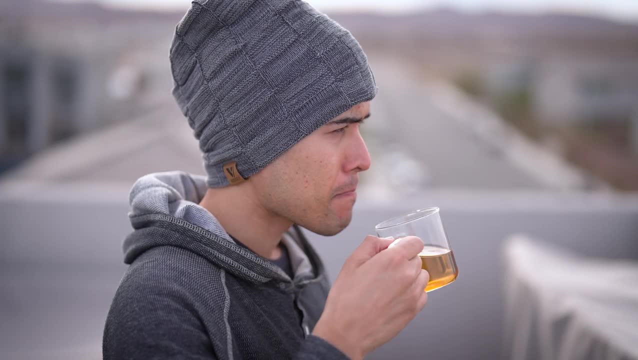 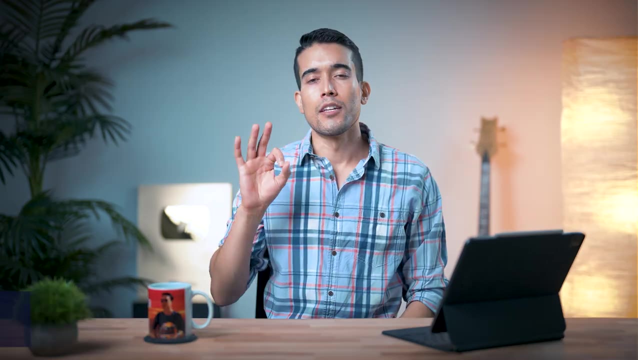 just stay hydrated. It's going to force you to go to the bathroom more regularly, and being hydrated is good for you, And the way to change that isn't by telling yourself to drink more water. It's by buying a water bottle and always keeping it on your desk. Number three is